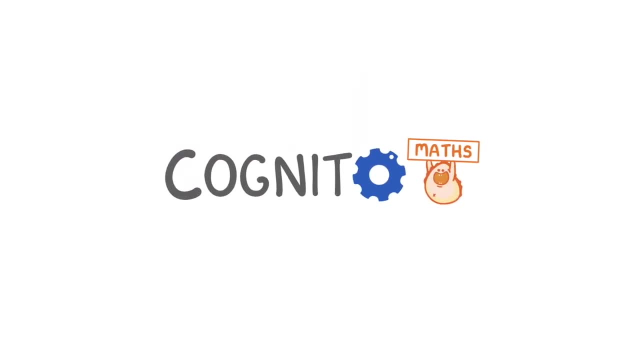 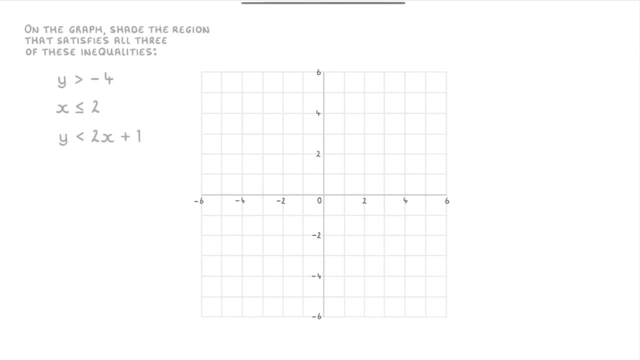 In this video we're going to cover how to do questions like this. We call these questions graphical inequalities and they require us to plot a bunch of inequalities on a graph. In this case, y is more than negative 4, x is less than or equal to 2, and y is less. 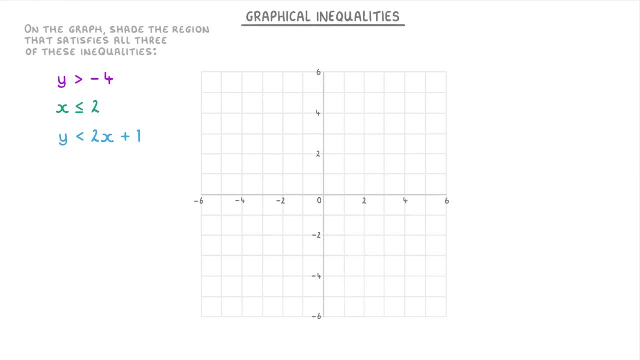 than 2x plus 1, and then find the region that satisfies all of them, And for this particular question, we're going to have to shade that region in To plot inequalities on a graph. you basically want to think of the inequalities as normal. 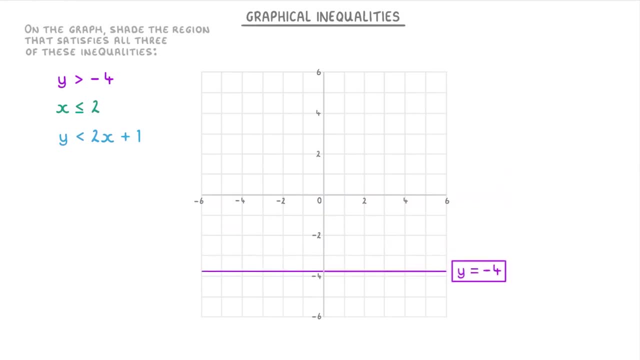 equations. so you just plot the lines: y equals minus 4, x equals 2, and y equals 2x plus 1.. If you can't remember how to plot lines on a graph, We've done a separate video on how to do it, so it might be worth checking that. 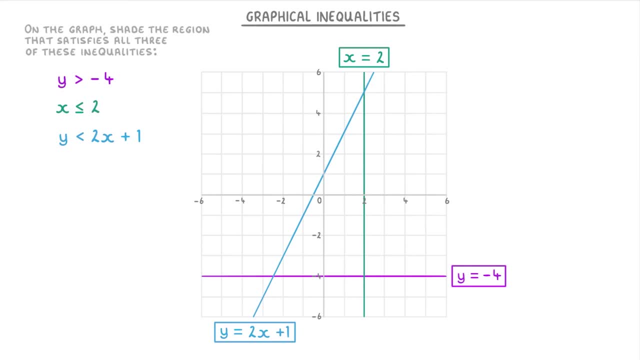 video out first. Now. one important difference is that if the inequality has a less than or a more than sign, you need to make the line dashed, But if it's a less than or equal to, or a more than or equal to, then we draw it with a solid line. 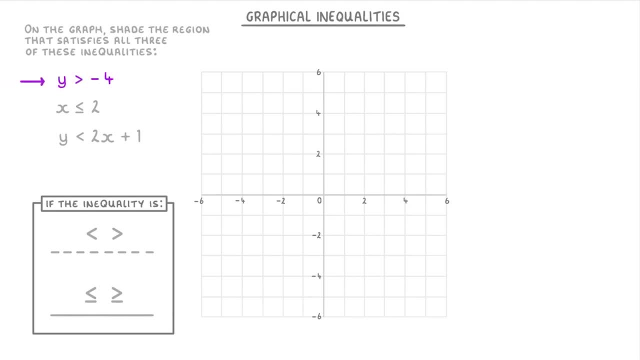 So if we go through this question properly and start with, y is more than negative 4, that would be a dashed horizontal line that crosses the y axis at negative 4.. And because our inequality tells us that y is bigger than negative 4, we know that the y value must. 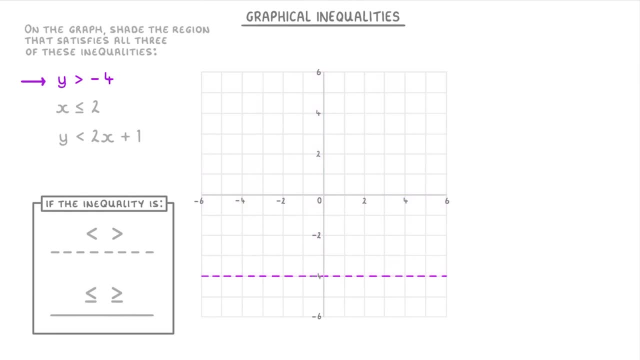 be on this side of the line, Because all of these y values like negative 2,, 0,, 2, and all the others are- are all big than negative 4.. In exams, a good tip is to draw two little arrows like this to: 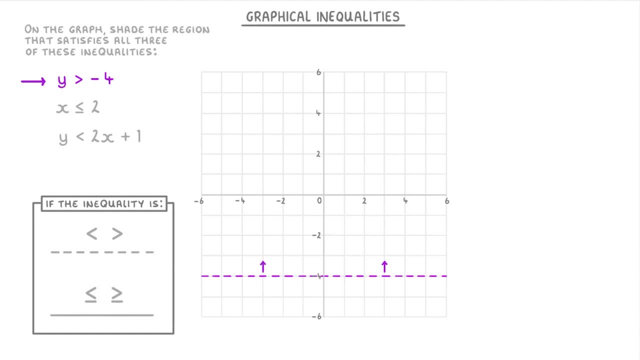 help remind you which side of the line you're looking at. Then, for our second inequality, x is less than or equal to 2, we draw a vertical line that cuts the x-axis at 2.. And remember, because it's a less than or, 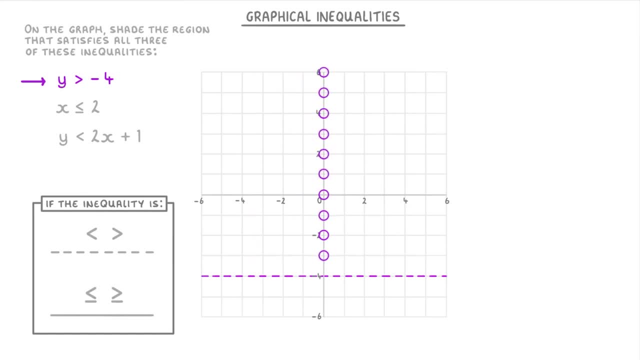 0,, 2 and all the others are all bigger than negative 4.. In exams, a good tip is to draw two little arrows like this to help remind you which side of the line you're looking at. Then for our second inequality, x is less than or equal to 2, we draw a vertical line. 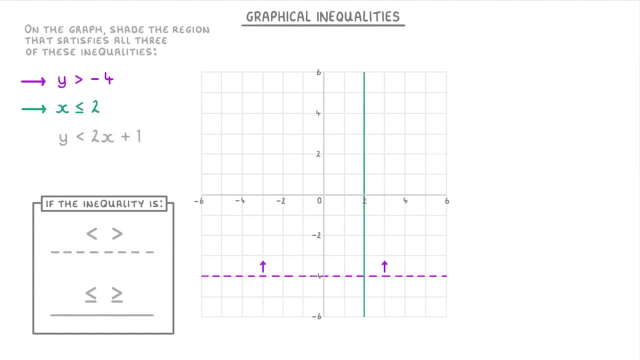 that cuts the x-axis at 2.. And remember, because it's a less than or equal to sign, the line needs to be solid, like this rather than dashed. And because it's less than or equal to 2, we know that the x-value will be somewhere. 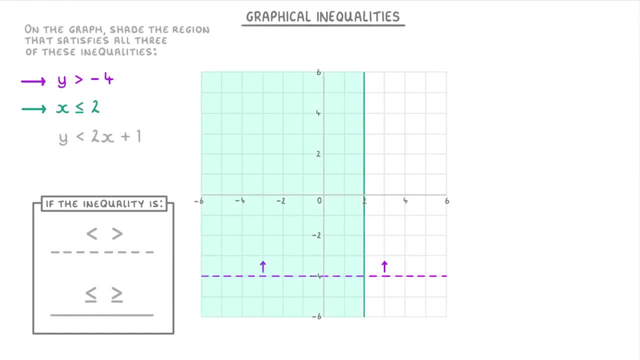 in this region to the left, where the x-values are all smaller than 2.. So we can draw our arrows on like this, pointing to the left. Finally, for y is less than 2x plus 1,, we draw a line that has a gradient of 2, and. 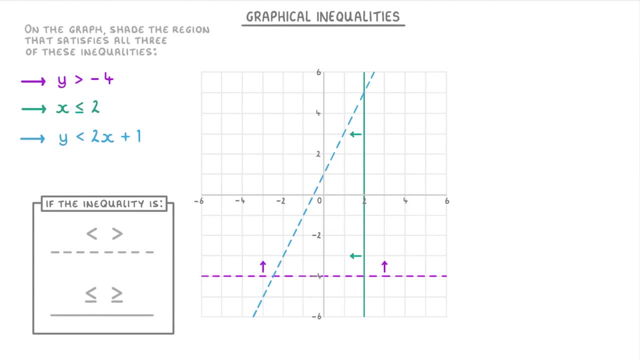 cuts the y-axis at positive 1.. And remember we have to draw it as a dashed line because it just has a less than sign. Figuring out which side of the line we're looking at is a bit trickier here, but basically, 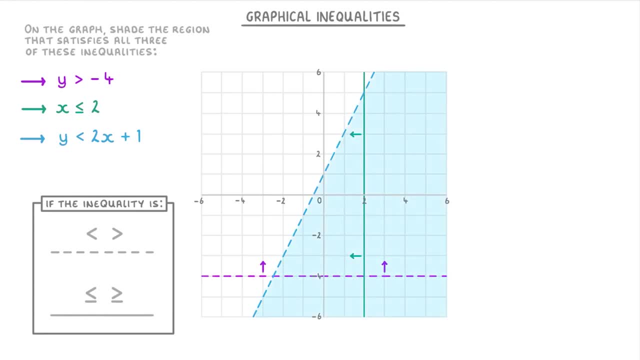 because it's a less than sign. we're looking at all the y-values that are lower than the line, So we can put little arrows pointing downwards. Also, I should point out that you won't get marks for the arrows in your exam. they're. 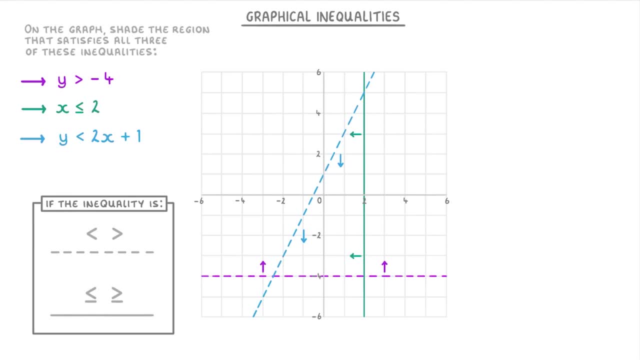 just a head Just to help you personally figure out which sides of the lines you're interested in. Then, to finish the question, we just need to shade the region that satisfies all the inequalities. So that means the region that's above our purple line but to the left of our turquoise. 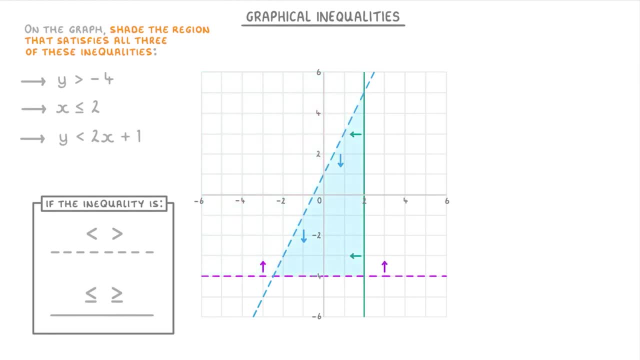 line and also below the blue line, Leaving us with just this little region in the middle as our answer- And this is how it normally works- You'll end up with a little area of the blue line that's above our turquoise line. You'll end up with a little area in the middle, in between all of the lines you've drawn. 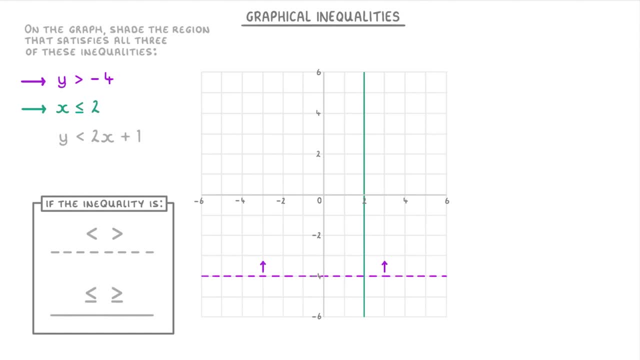 equal to sign. the line needs to be solid like this rather than dashed. And because it's less than or equal to 2, we know that the x-value will be somewhere in this region to the left where the x-values are all smaller than 2.. So we 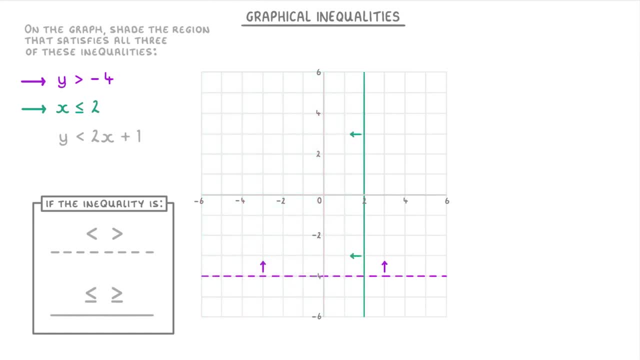 can draw our arrows on like this, pointing to the left. Finally, for y is less than 2x plus 1, we draw a line that has a gradient of 2 and cuts the y-axis at positive 2.. And remember, we have to draw it as a dashed line because it just has a less than sign. 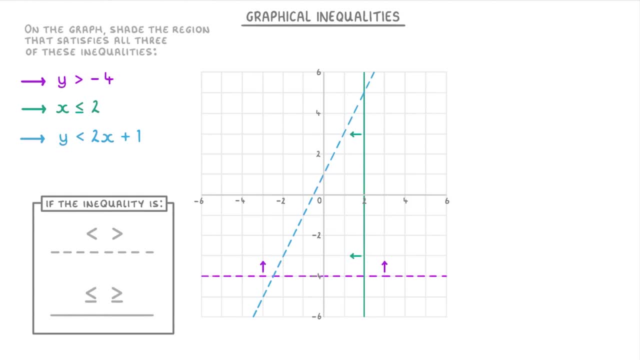 Figuring out which side of the line we're looking at is a bit trickier here, But basically because it's a less than sign, we're looking at all the y-values that are lower than the line, So we can put little arrows pointing downwards. Also, I should point out that you 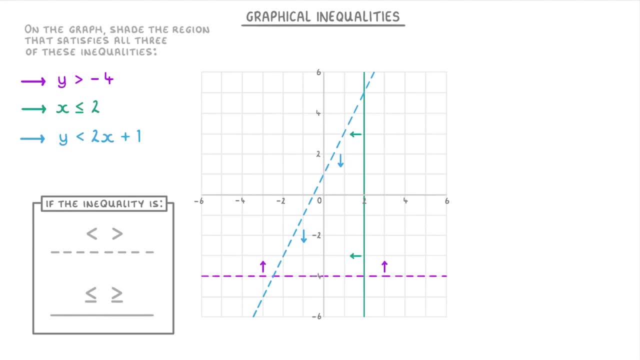 won't get marks for the arrows in your exam. They're just to help you personally figure out which side you're looking at. Then, to finish the question, we just need to shade the region that satisfies all the inequalities, So that means the region that's above our purple line but to the left of 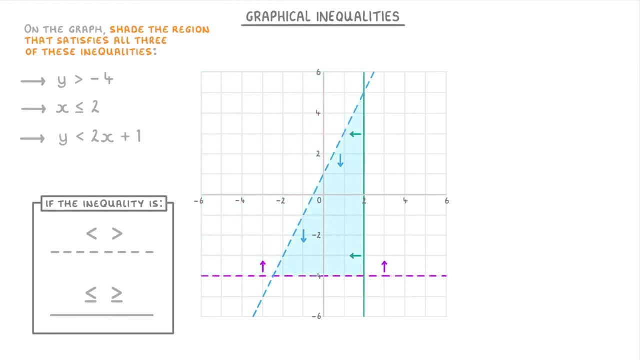 our turquoise line and also below the blue line, Leaving us with just this little region in the middle as our answer- And this is how it normally works- You'll end up with a little area in the middle, in between all of the lines you've drawn, So it's normally pretty easy to spot. 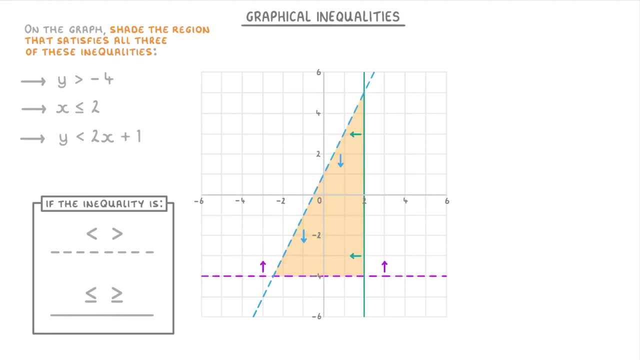 Something else to point out is that, instead of being asked to shade the region, you might sometimes be asked to label the region in some way. For example, label the region that satisfies all three of the inequalities with the letter R. So in that case, you'd just 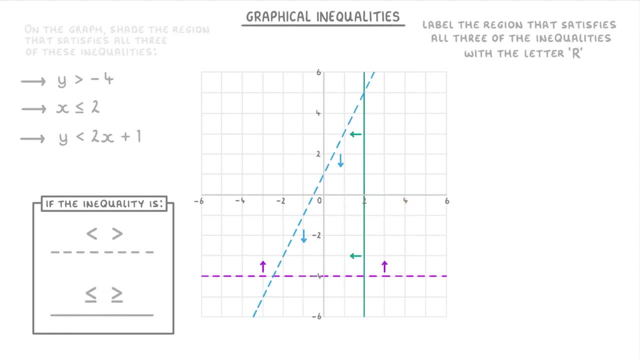 put a big R in there. Alternatively, you could be asked to mark all of the points that are satisfied, So for that you'd have to put little crosses on all of the points inside the area. Importantly, though, because x is less than or equal to 2, we also need to put 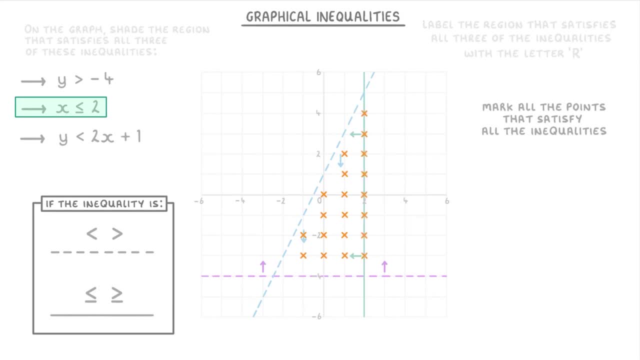 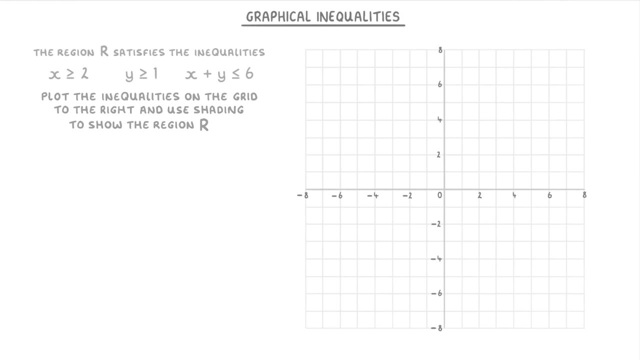 crosses on these points, because the x value can also be 2 itself. Let's quickly have a go at one more before we finish. This question says that the region R satisfies all three of the points in the area. It satisfies the inequalities: x is more than or equal to 2, y is more than or equal to. 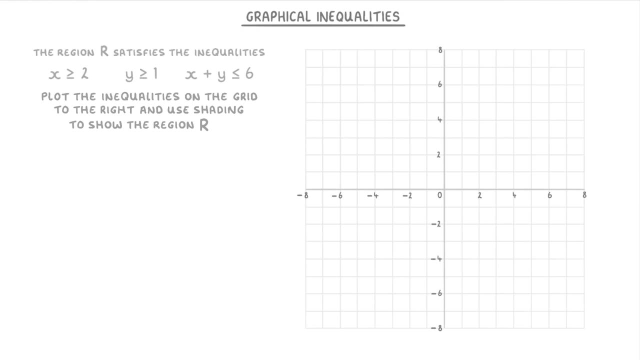 1, and x plus y is less than or equal to 6.. And it then asks us to plot the inequalities on the grid to the right and use shading to show the region R. So the first thing that we want to do here is draw out our lines with their little arrows on: So x equals 2, with. 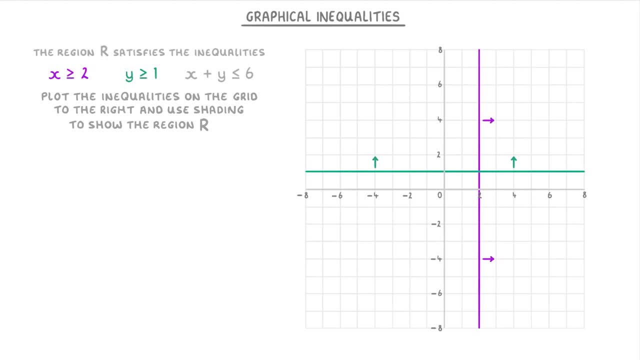 arrows to the right, y equals 1, with arrows upwards, And x plus y equals 6, with arrows downwards. And now that we have all of our inequalities, we just need to find the region that satisfies all of them. So, to the right, of x equals 2,, above, y equals 1, and below, x plus y equals 6.. And 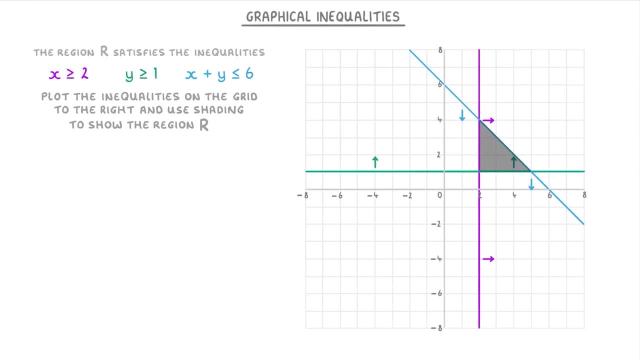 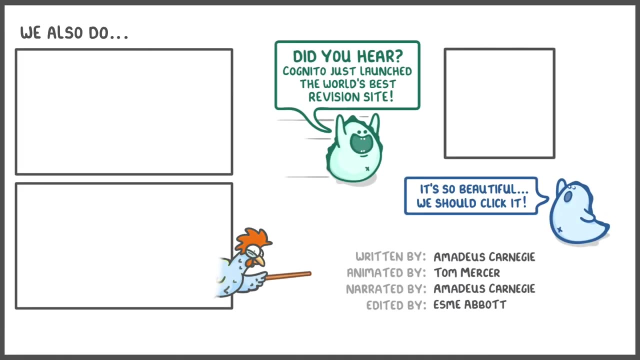 now that we've found it, we just shade it in And we're done. That's everything for this video, though, So if you found it useful, then please do tell your friends and teachers about us, And thanks for watching. 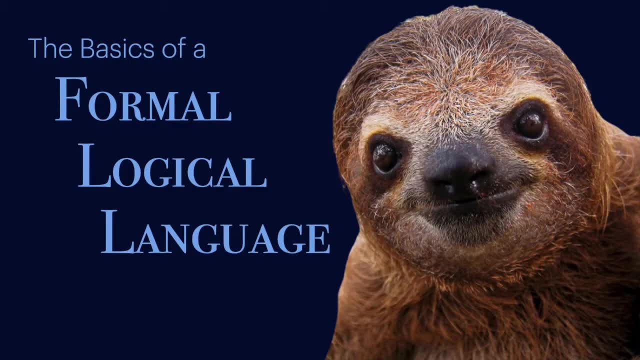 Natural languages like English or Spanish are dynamic and fluid, full of nuance and ambiguity. That's great for poetry, not so great for logic. For the clarity and precision logic demands, 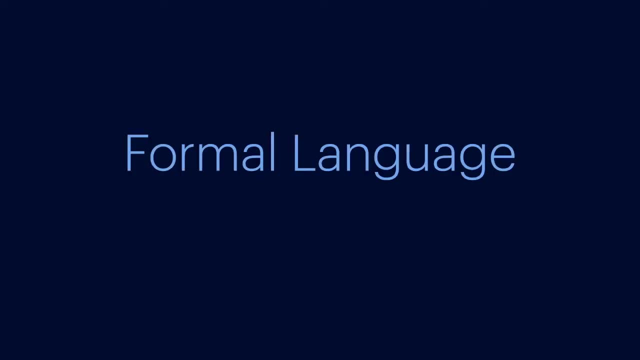 we must turn to a formal language, that is, an artificial symbolic language built with one purpose in mind, to express complex logical ideas simply. Here's an example. This might look 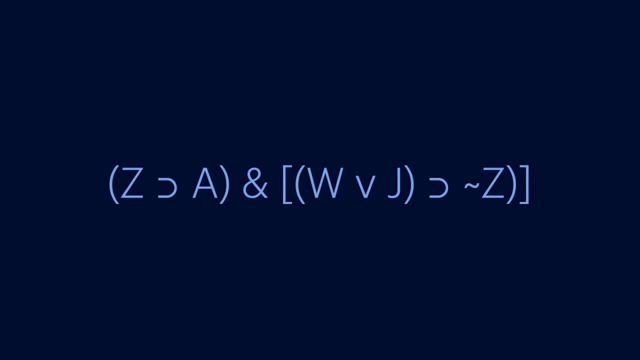 confusing now, but with a little practice, it's a huge improvement over the same sentence written in English. Now, maybe you've had a bad experience in math, and your heart rate goes up when you see a symbolic formula like this. But stick with me. Almost anyone can master the basics of a formal logical language. In fact, there are only three elements that make up a sentence of